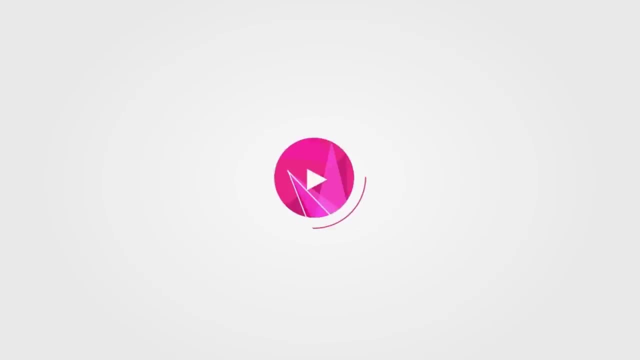 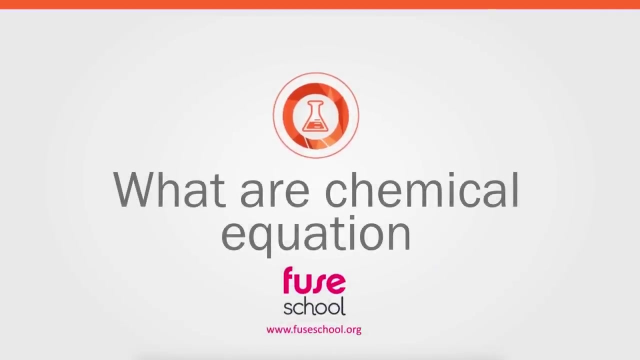 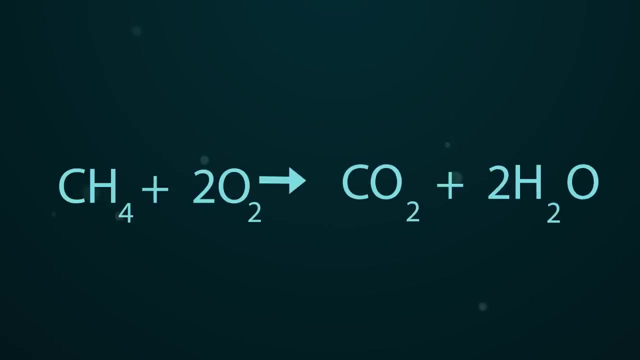 Chemical equations can sometimes look a bit daunting, especially when there are lots of different compounds and state symbols involved. but fear not to help in this lesson about chemical equations. Quite simply, a chemical equation shows the overall chemical change of reactants into products. It's a bit like a detailed 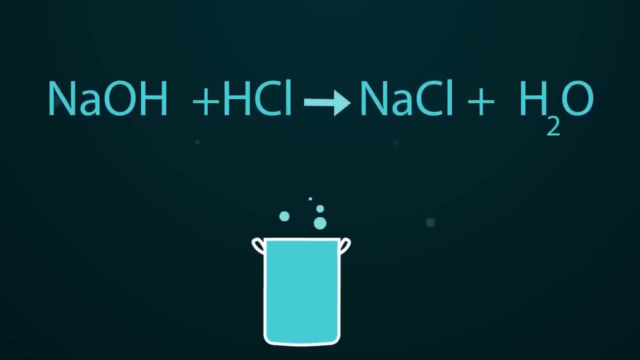 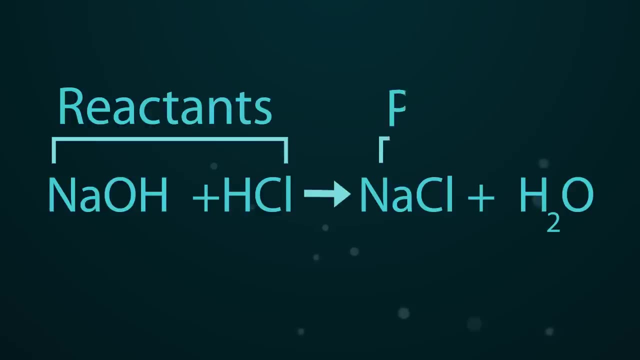 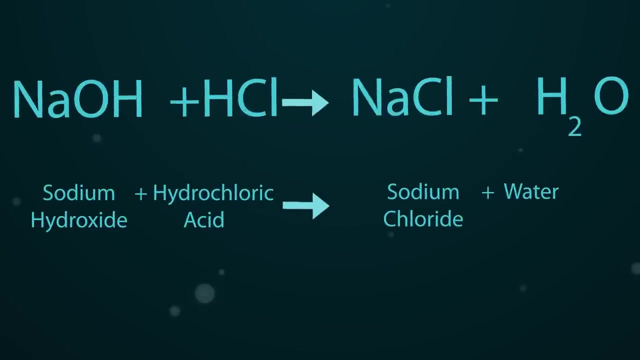 cooking recipe, but where all the ingredients and all the products are written down, even the ones you can't necessarily see. The reactants are what you start with and the products are what are formed. There are two ways of writing chemical equations: word equations and symbol equations. When they are written, 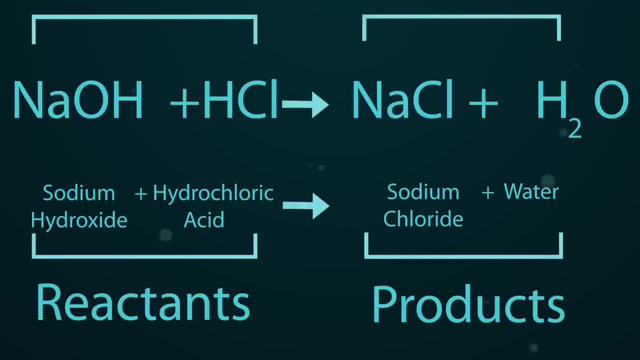 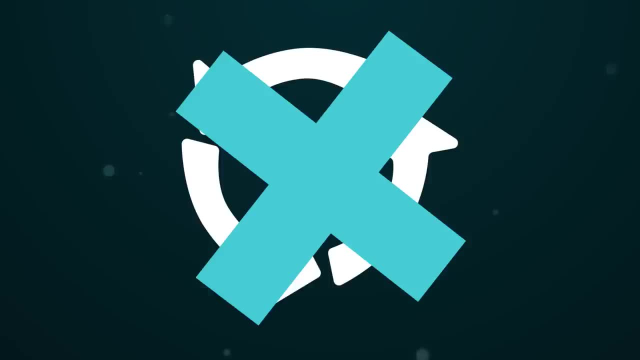 both types show the reactants on the left of an arrow and the products on the right. The arrow is there to show that the reaction is irreversible. If you like, it shows the direction of the reaction and that it is one way, a bit like a one-way. 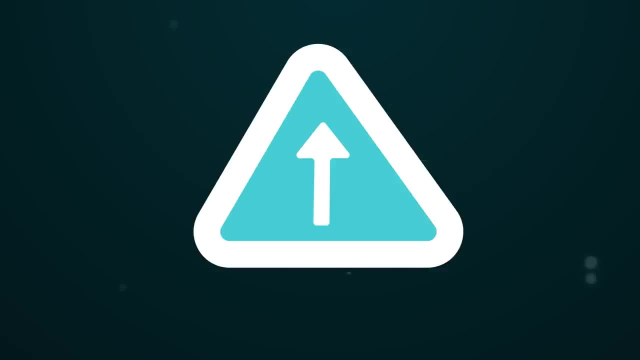 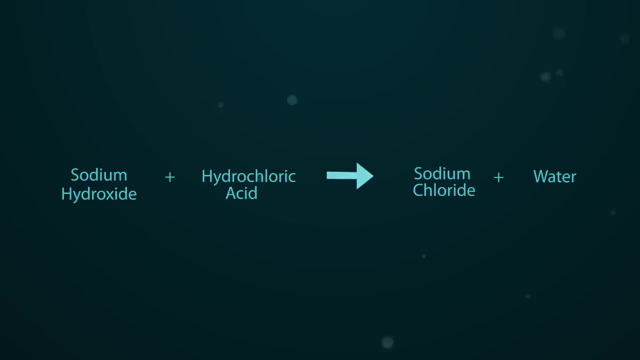 street. You can't reverse along a one-way street and you can't reverse an irreversible reaction. Let's look at a word equation. This is a way of summarizing a chemical reaction, For example, the neutralization of hydrochloric acid with sodium hydroxide. We would write sodium hydroxide. 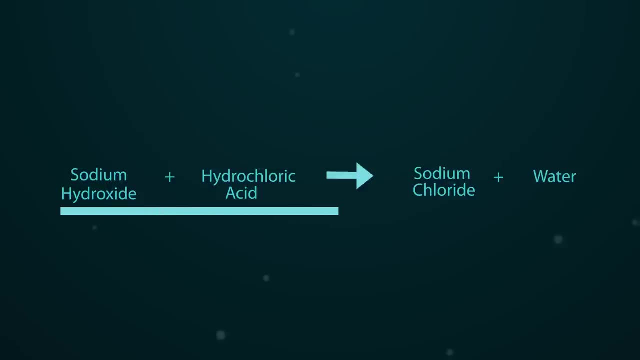 plus hydrochloric acid, then the arrow sodium chloride plus water. The plus sign indicates that there is more than one reactant or product on each side of the equation, and you'll note that the reactants are on the left and the products are on the right. We've also written this all on a single line. It. 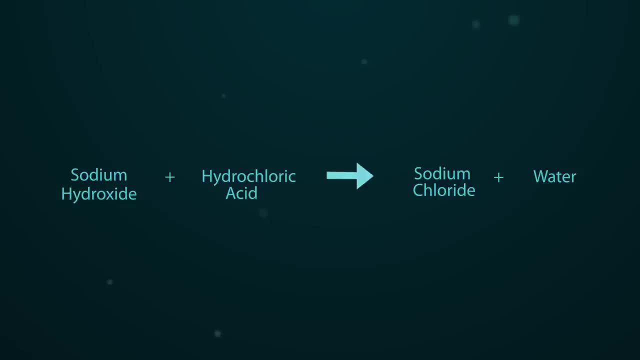 makes it a lot easier to read this way. So when you write your equations, try to keep all of the information on a single line. If you can't, then the arrow becomes an important separator. The rule of reactants on the left and product on the right still applies because if not, the 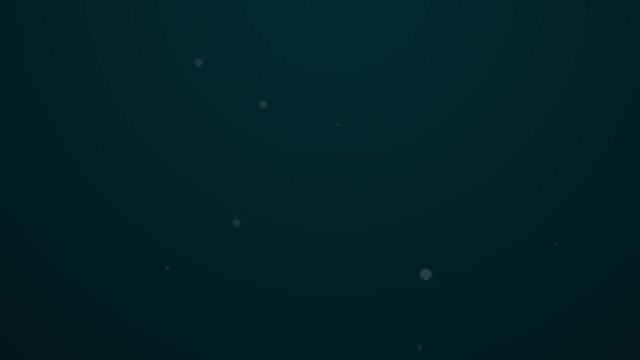 equation can become a jumbled mess. A clearly written equation is always easier to understand. A word equation provides a good summary, but a symbol equation provides more information. It shows more detail and allows us to see how many atoms and molecules are involved in each one.